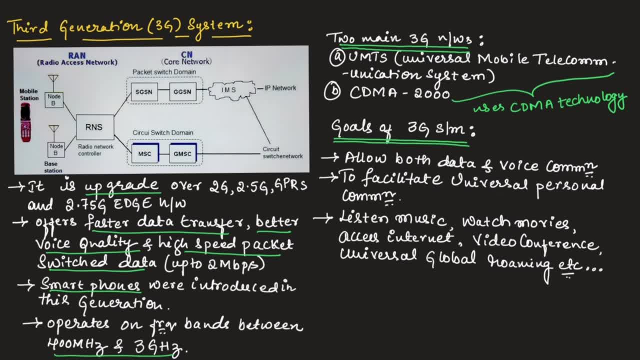 So it also facilitates the universal personal communications between the user. These 3rd generation systems are very much helpful for listening music, watching movies, access to internet, video conference, universal global roaming, etc. So these are the different applications of 3rd generation systems. 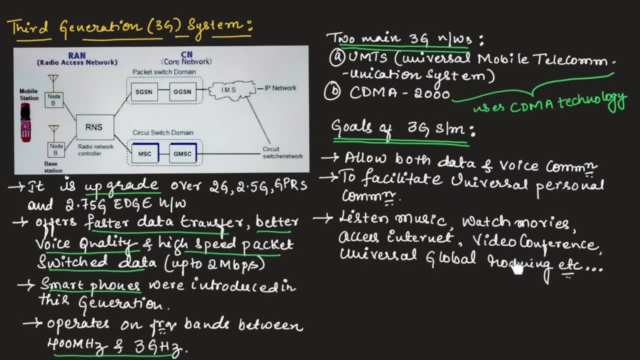 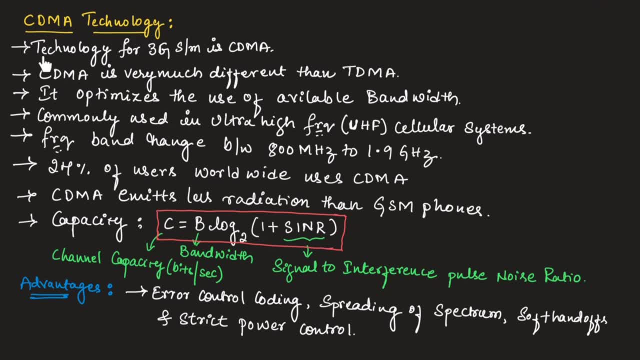 Our 2nd generation system, in which these are all not possible. Now let us understand CDMA technology. The dominant technology or main technology that is used for 3rd generation system is CDMA. So the main technology that is used for 3rd generation system is CDMA. 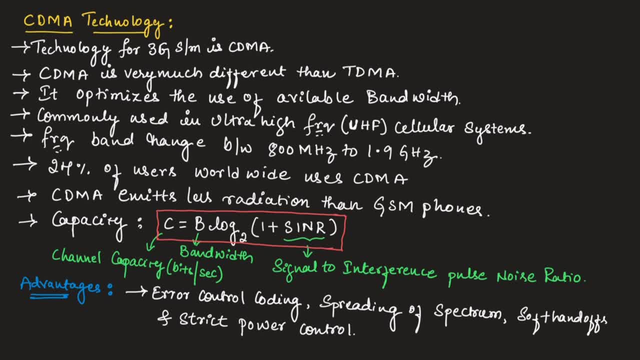 So the main technology, or main technology that is used for 3rd generation system is CDMA. CDMA is very much different than TDMA. So we understood this in our previous lecture, where we understood that CDMA is different than TDMA. 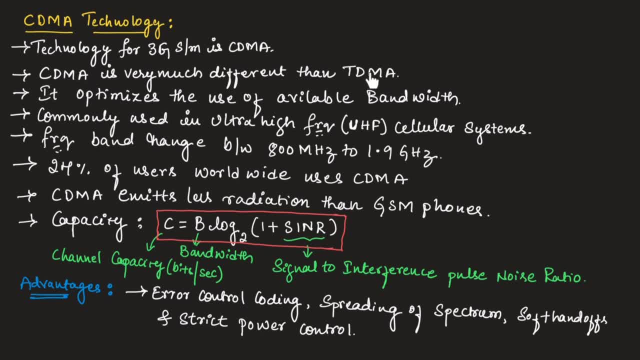 So CDMA is code division- multiple access- and TDMA is time division- multiple access. CDMA optimizes the use of available bandwidth, So it will optimize the available bandwidth, which means it will make use of available bandwidth. This technology is commonly used in ultra high frequency cellular system. So this is most commonly used in UHF cellular system, which is ultra high frequency cellular systems. The frequency band range of CDMA is ranging between 800 megahertz to 1.9 gigahertz, So the frequency will range between 800 megahertz to 1.9 gigahertz. 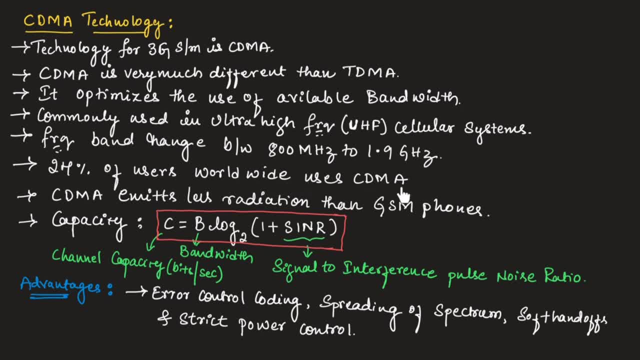 24% of users worldwide use CDMA. So this is very less compared to GSM technology, But, as you can see here, 24% of users worldwide use CDMA technology. So most of the users worldwide uses GSM technology. 24% of the users will use CDMA technology. 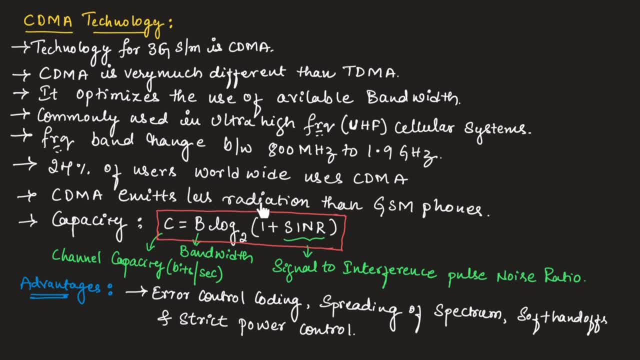 So CDMA technology emits less radiation when it is compared with GSM phones, So CDMA phones will emit less radiation compared to GSM phones. So here channel capacity is very important. The capacity of mobile telecommunication system in CDMA technology can be given as: